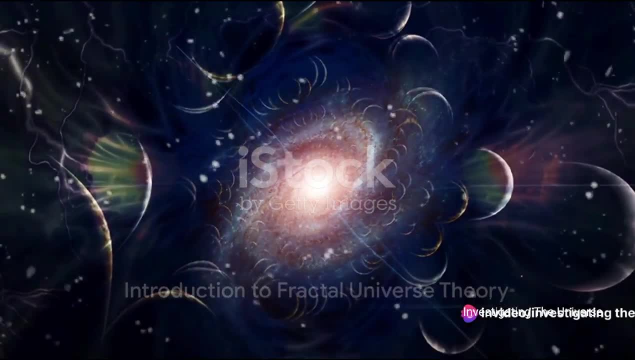 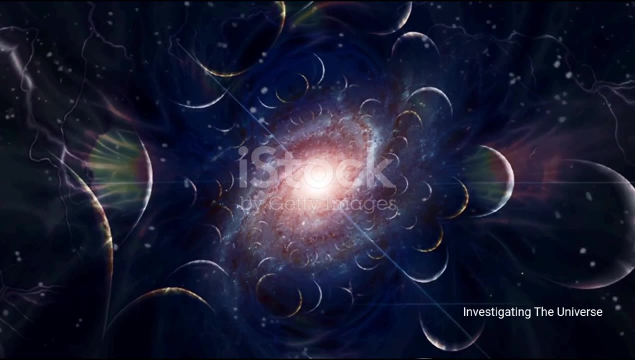 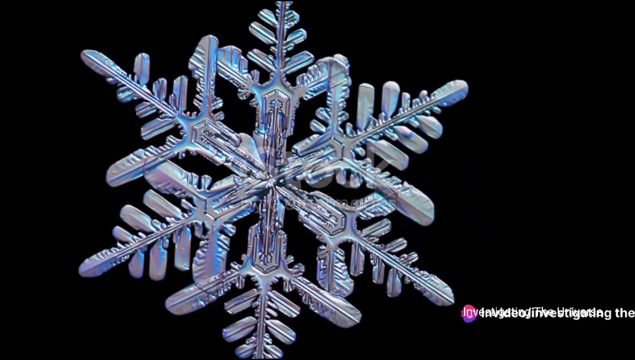 Welcome to Investigating the Universe, where we unravel the mysteries of the cosmos. Today, we're embarking on a journey to explore one of the most intriguing theories in modern cosmology: the fractal universe theory. Picture a snowflake: Its intricate design is formed of 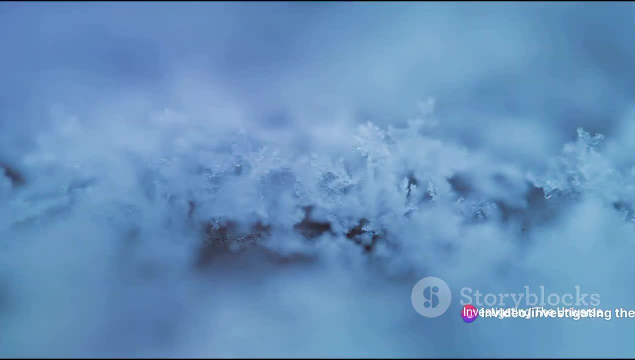 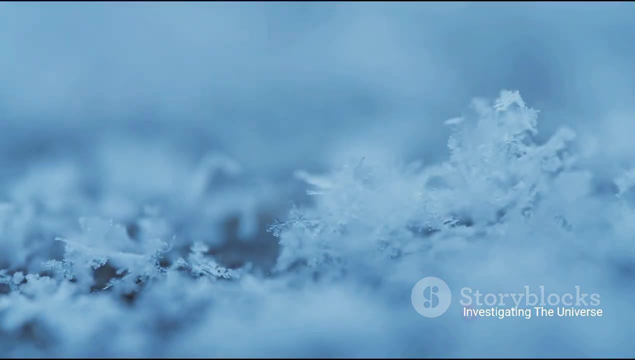 smaller versions of itself, repeated over and over again. This self-similar pattern, seen across different scales, is known as a fractal. Now imagine applying this concept to the universe. Could the cosmos be an infinite, ever-repeating pattern? a cosmic fractal of? 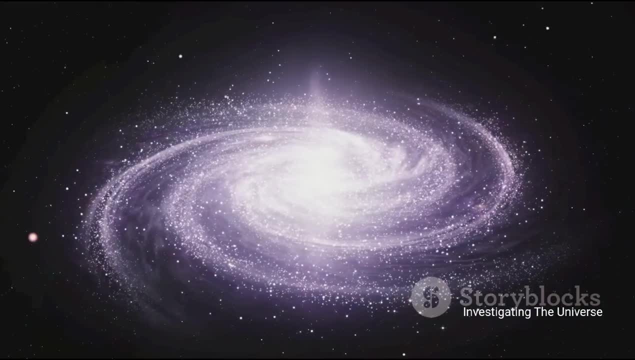 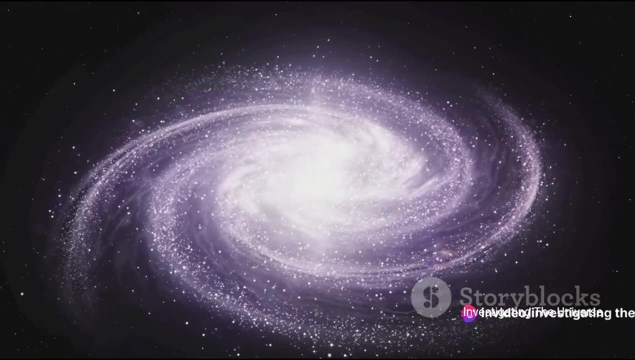 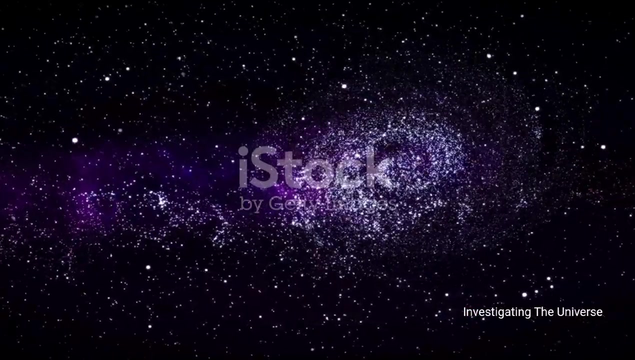 galaxies, stars and planets. This is the core idea behind the fractal universe theory, a concept suggesting that the universe's structure isn't just random, but follows a fractal pattern. It's a captivating thought, isn't it A universe where everything from the 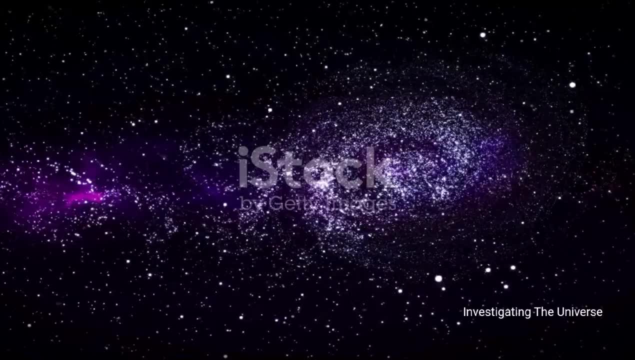 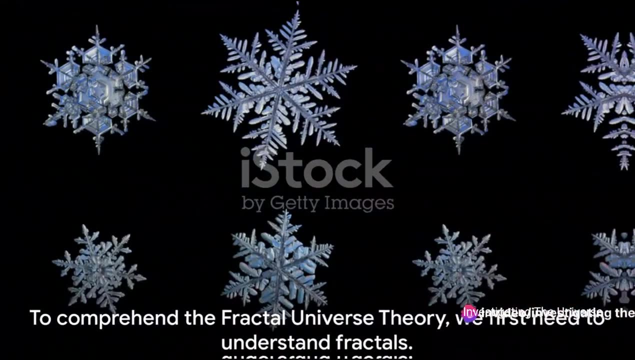 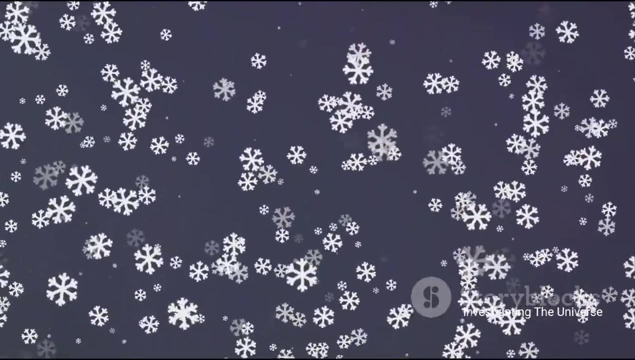 tiniest particle to the largest galaxy could be a part of a grand repeating pattern. Now let's dive deeper into the concept of fractals. To comprehend the fractal universe theory, we first need to understand fractals. So what are fractals? Picture a snowflake in. 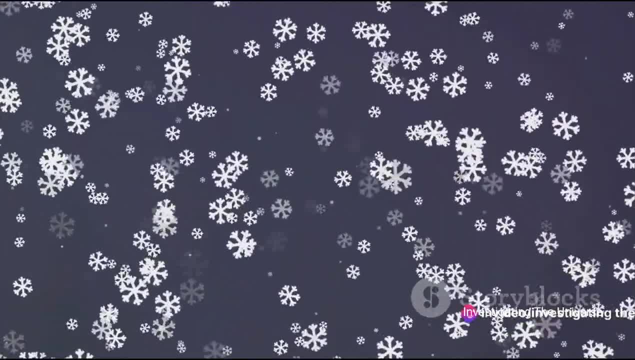 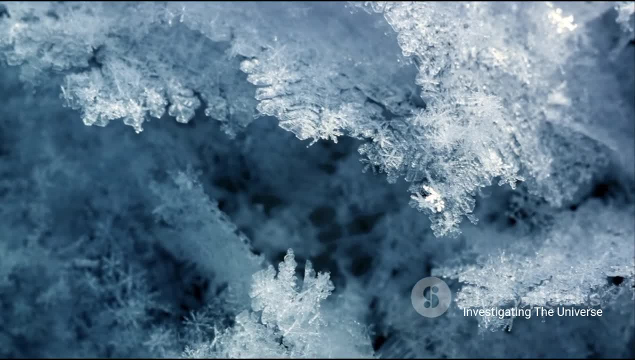 your mind. Each arm of the snowflake is a miniature version of the whole. No matter how much you zoom in, you'll find the same pattern repeating over and over again. This is the essence of a fractal, an object or pattern that is self-similar across different scales. 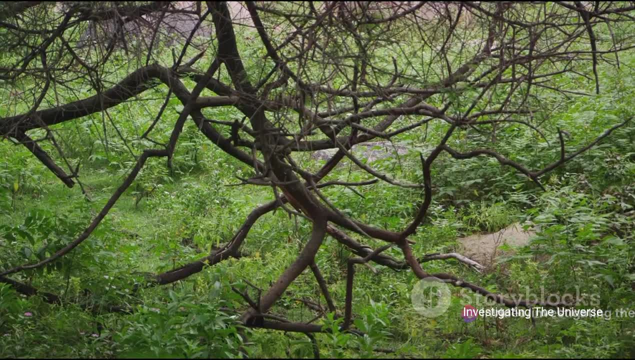 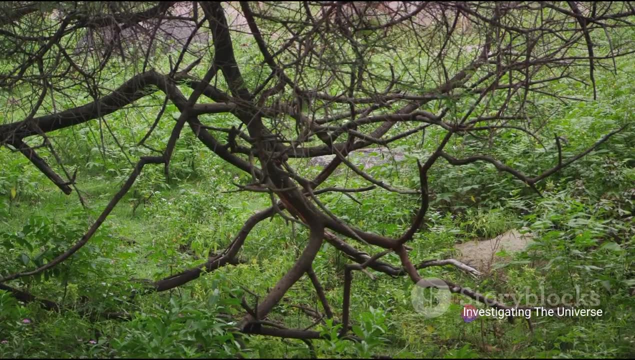 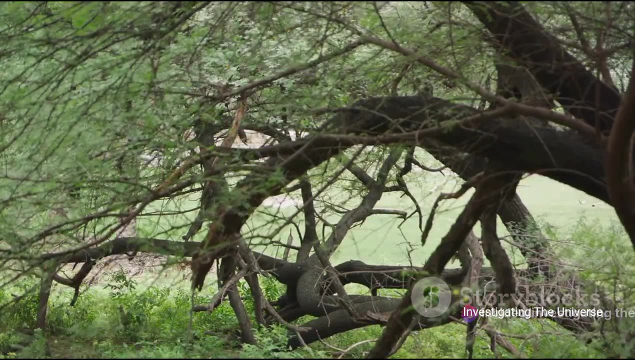 Fractals are not just limited to snowflakes. They can be found all around us in nature. Consider the branches of a tree. Each branch divides into smaller branches, which further divide into even smaller branches, and so on. Each level of branching is a smaller-scale replica of 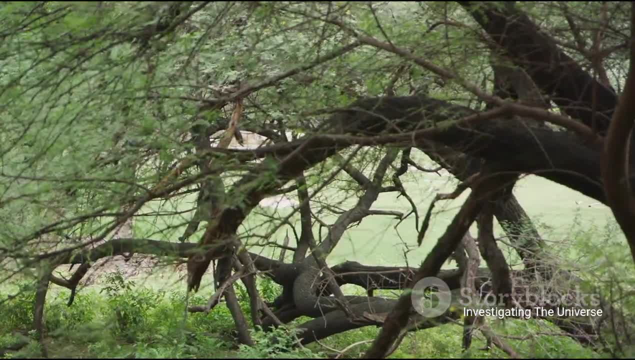 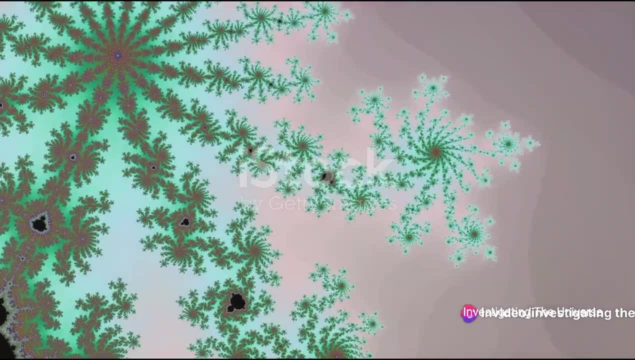 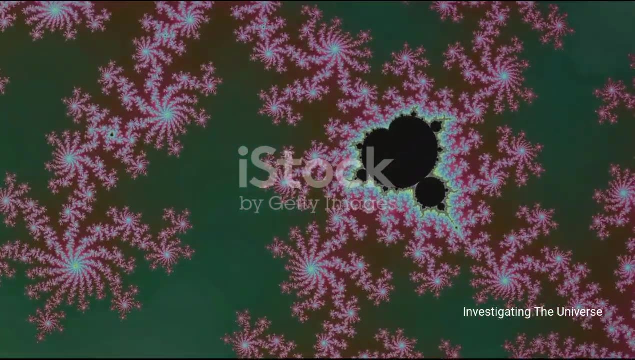 the whole tree. Similarly, river networks with their tributaries and subtributaries also exhibit fractal structures. But fractals are not just confined to physical objects. They can also be mathematical constructs, like the famous Mandelbrot set. It's a set of complex. 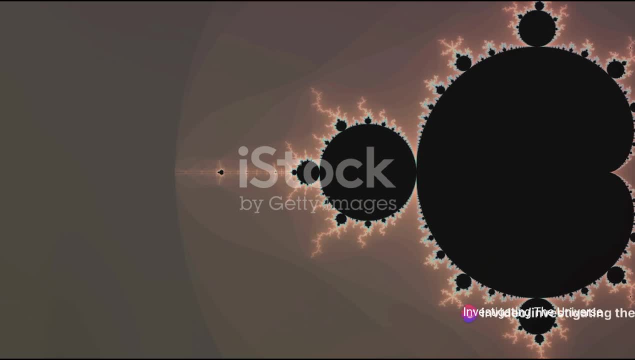 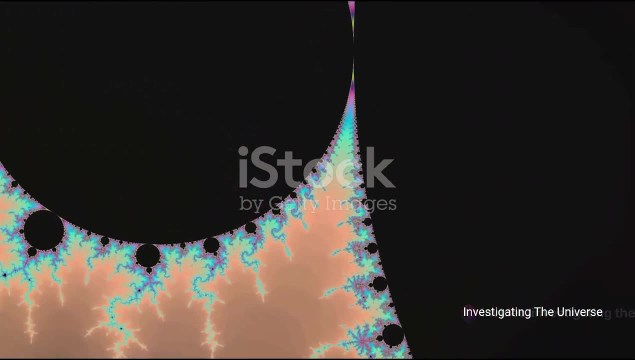 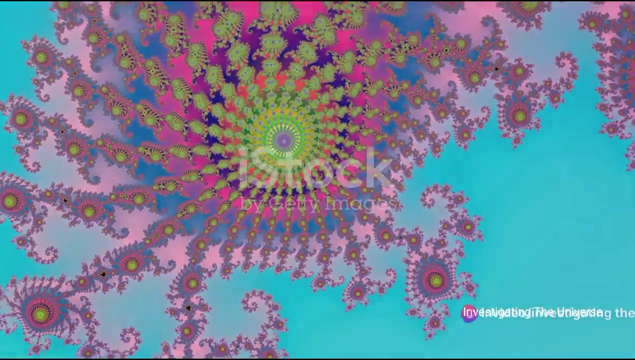 numbers, that generates a mesmerizing fractal pattern when plotted on a plane. With each zoom, the pattern continues to reveal more intricate details, But the overall shape remains the same. In essence, a fractal is a pattern that repeats at every scale. It's a concept that blends the 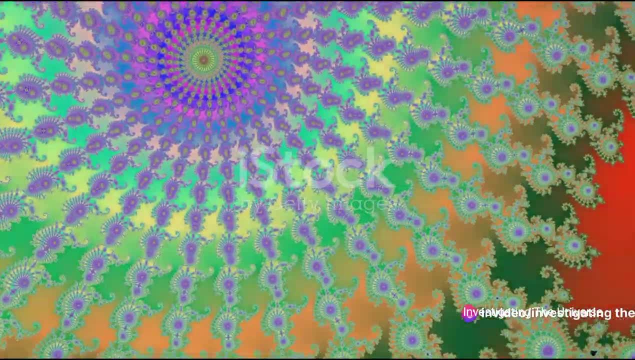 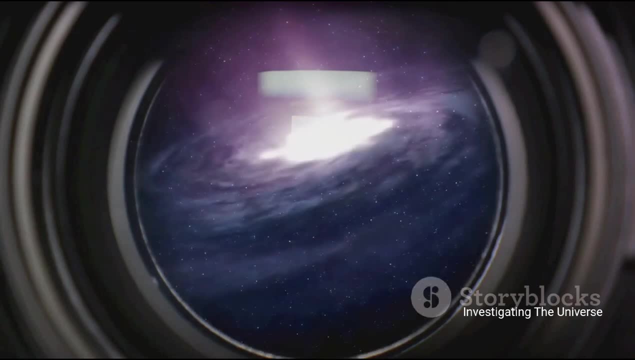 finite and the infinite, the simple and the complex. This idea of self-similarity across scales is what makes fractals so fascinating. But why are we talking about fractals in a discussion about the universe? Well, the fractal universe theory proposes that the structure of the 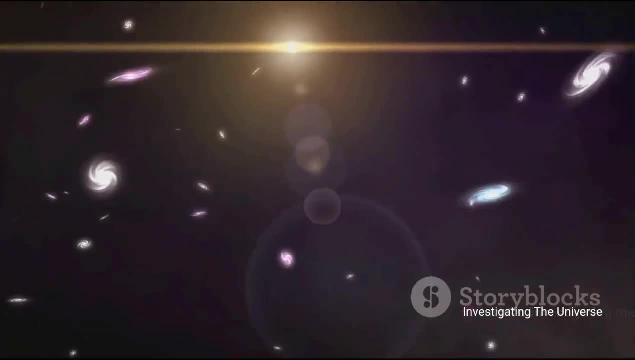 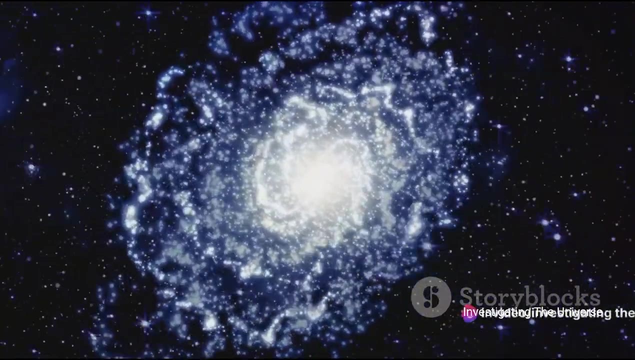 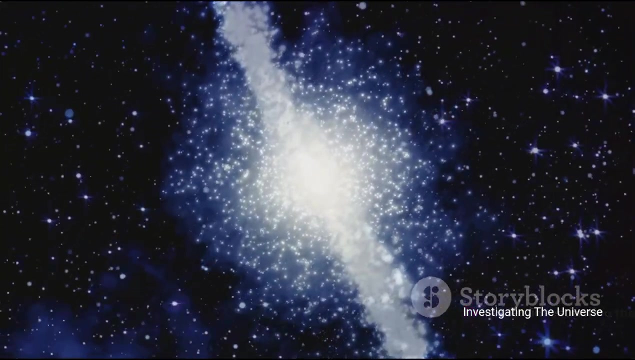 universe itself is fractal-like. Just as a tree branch is a smaller-scale version of the whole tree, each galaxy could be a smaller-scale version of the entire universe. With this understanding of fractals, we can begin to explore how this concept applies to our universe. 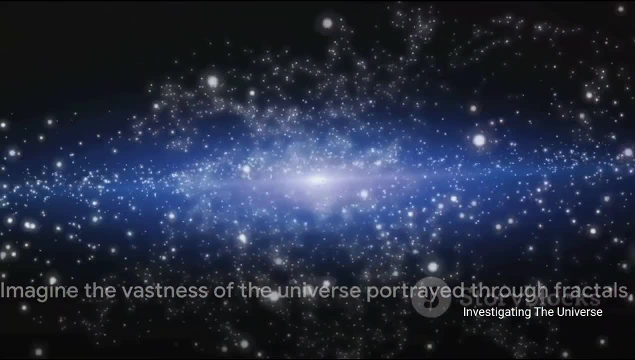 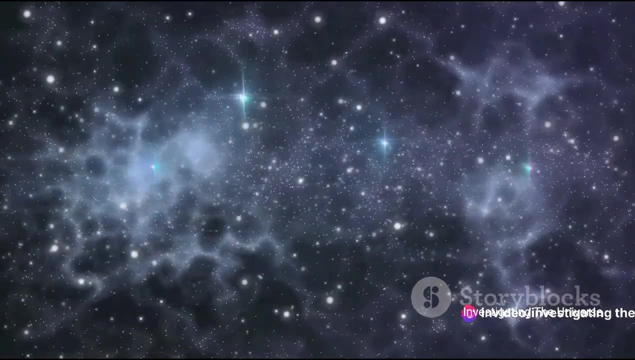 Now imagine applying this concept of fractals to the entire universe. That's right. the idea of fractals isn't confined to the realm of mathematics or the intricate designs in a kaleidoscope. It extends far beyond, into the vast expanses of the cosmos. This is what the fractal universe. 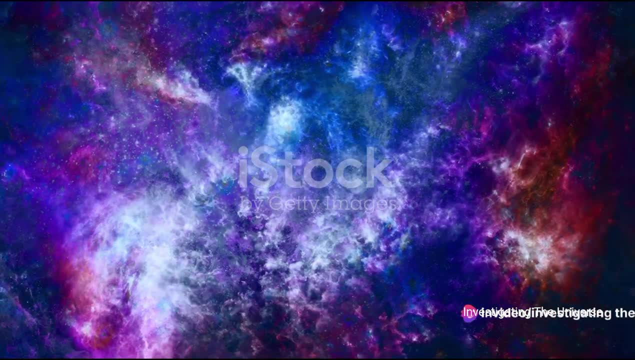 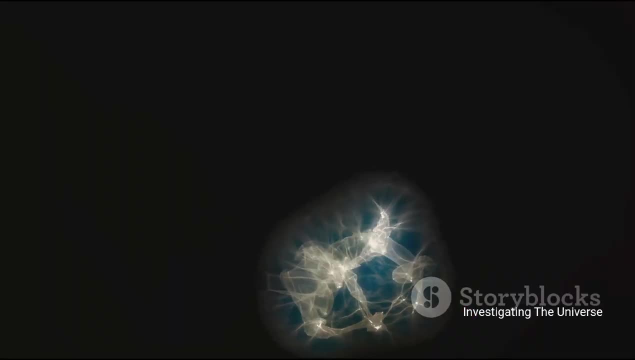 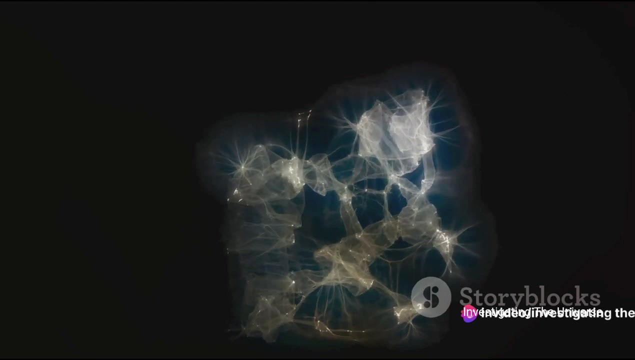 theory proposes. It suggests that the universe, in its infinite complexity, also follows the patterns of fractals. To understand this, let's consider the large-scale structure of the universe. When we gaze at the night sky, we see a seemingly random array of stars and galaxies. Yet 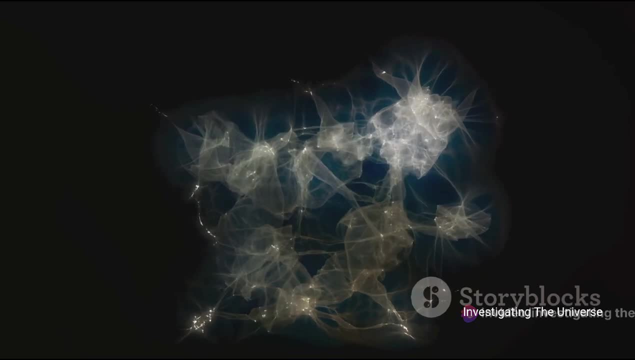 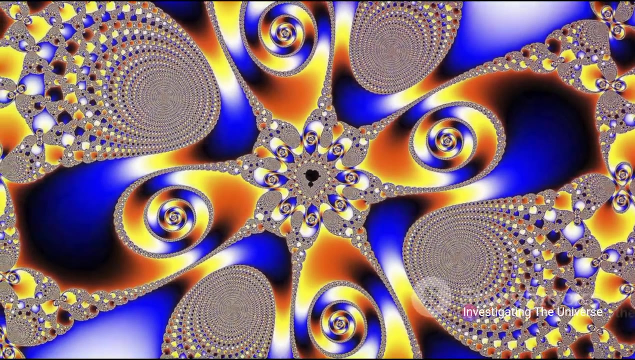 as scientists have delved deeper, they've found patterns emerging from this apparent chaos. Galaxies, it turns out, are not just randomly scattered across the universe. They form clusters, And these clusters come together to form superclusters And these superclusters. They are part of even larger structures. It's a pattern of patterns, a hierarchy of structures, Much like a fractal. each part of the universe appears to mirror the whole, regardless of scale. But it's not just about the physical placement of celestial bodies. 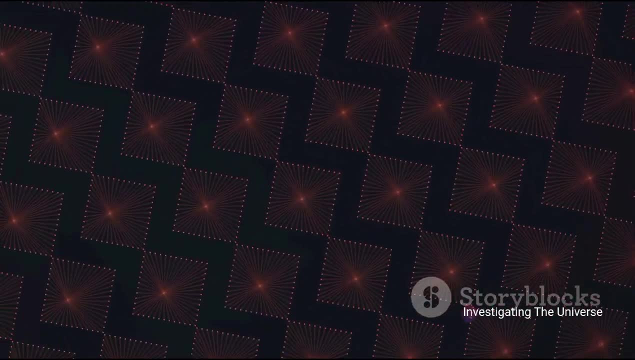 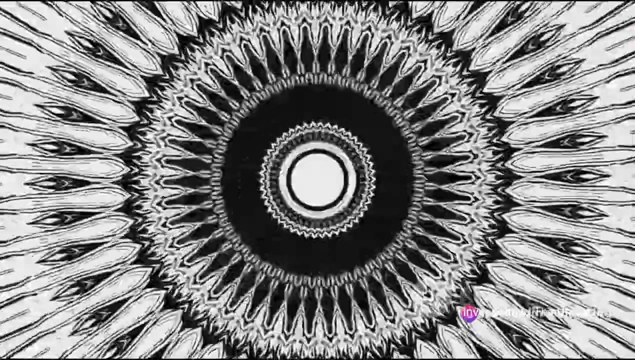 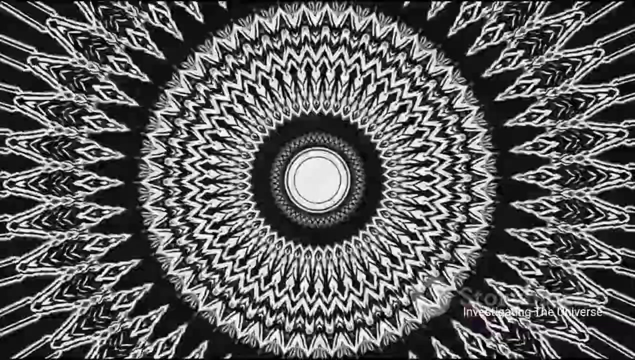 The fractal nature of the universe can also be seen in the cosmic microwave background radiation, the afterglow of the Big Bang. This radiation is not uniform, but rather shows slight variations in temperature. These variations appear to follow a fractal pattern. 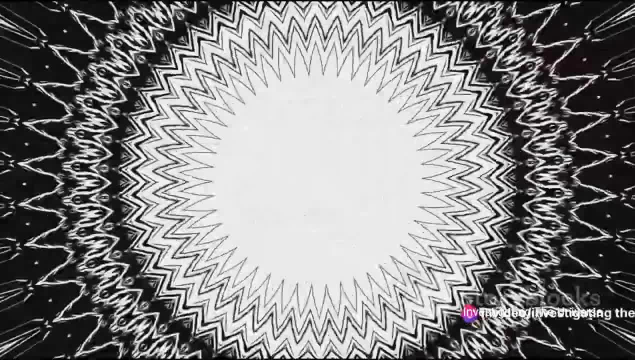 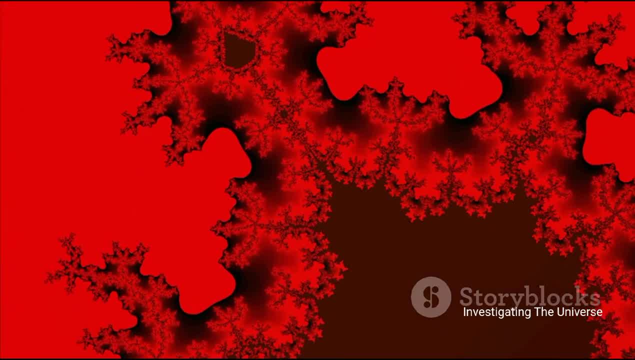 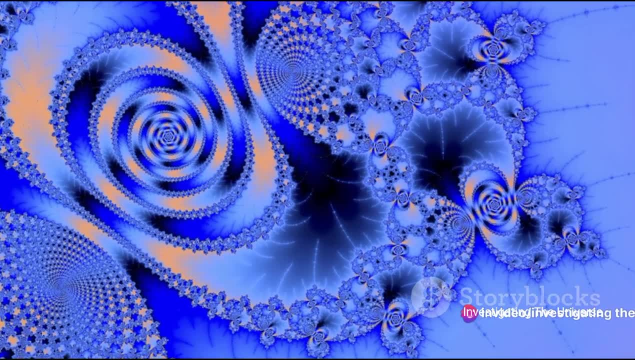 allowing us to follow the universe. but they alsogee on the Earth's surface, which is practically never really visible, And that's another piece of the puzzle in our understanding of the universe's structure. The fractal universe theory paints a picture of the cosmos as an ever-repeating pattern, A cosmic fractal, if you will. It implies an 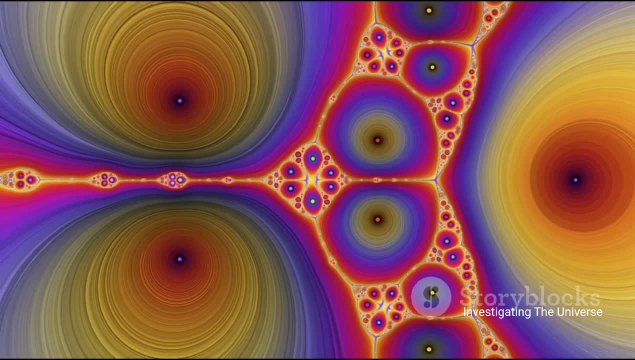 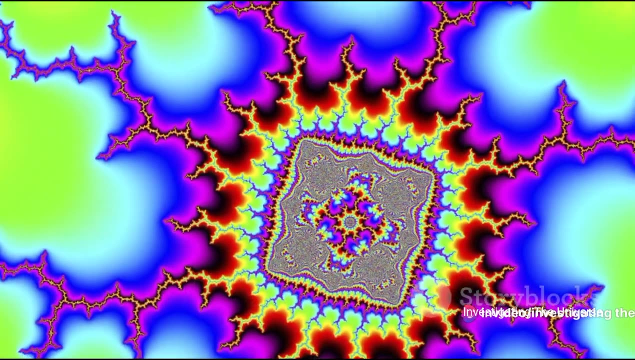 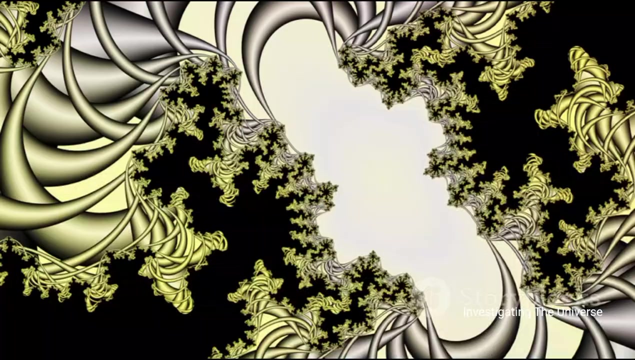 inherent order within the seeming disorder of the universe, an endless dance of creation and destruction, of galaxies being born and dying, all following a fractal pattern. It's a fascinating vastness and complexity could be boiled down to a simple recurring pattern, a pattern that we can find in the veins of a leaf, the branches of a tree or the 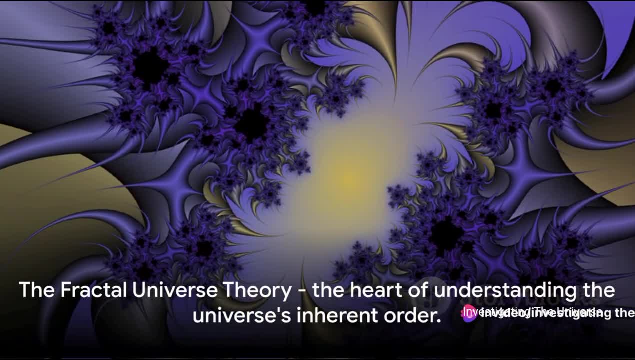 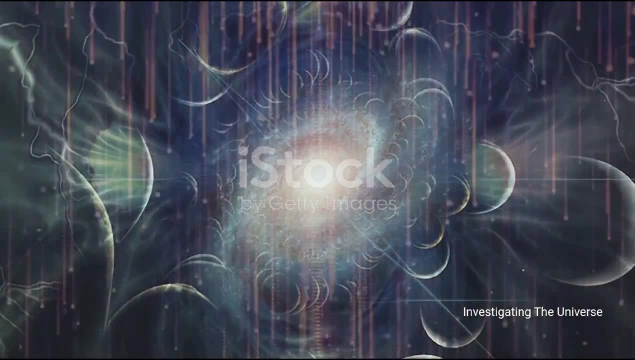 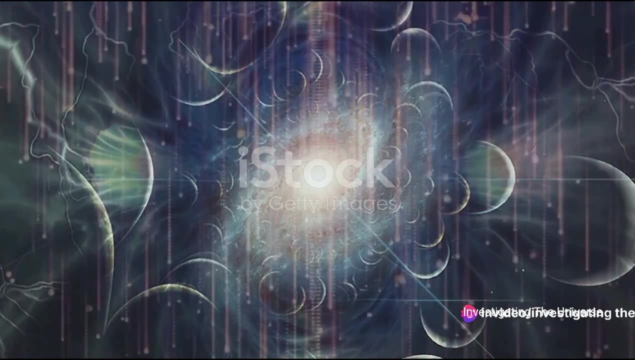 spirals of a seashell. this concept is at the heart of the fractal universe theory. you might wonder what evidence supports this theory. well, there are two main pieces of evidence that support the fractal universe theory. the first comes from the large-scale structure of the universe itself. when we look out into 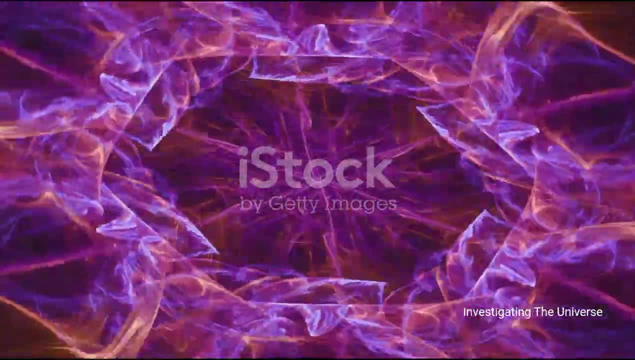 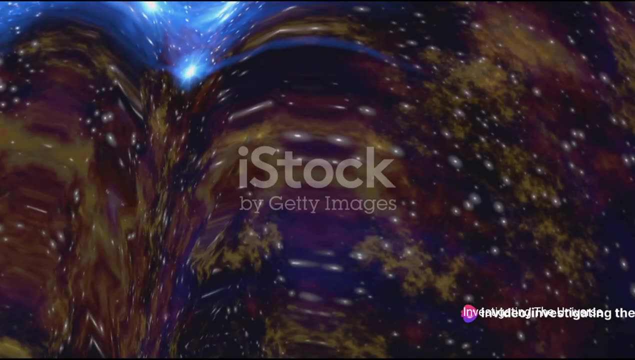 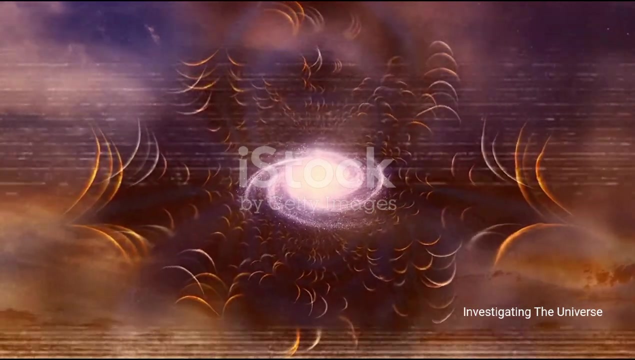 the cosmos with our high-powered telescopes, we see a universe that is far from uniform. instead, it's a vast cosmic web of galaxies, each one interconnected in a complex pattern that spans the entire observable universe. these patterns, upon closer examination, reveal a remarkable similarity to fractal. 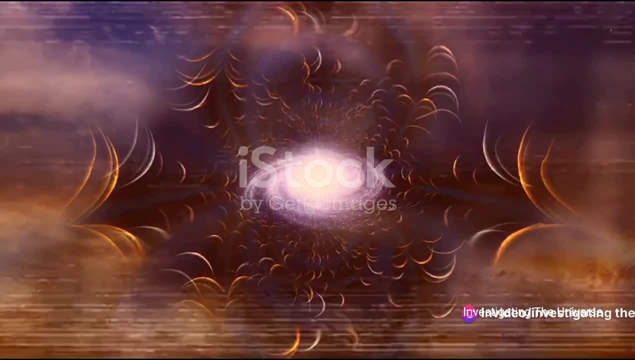 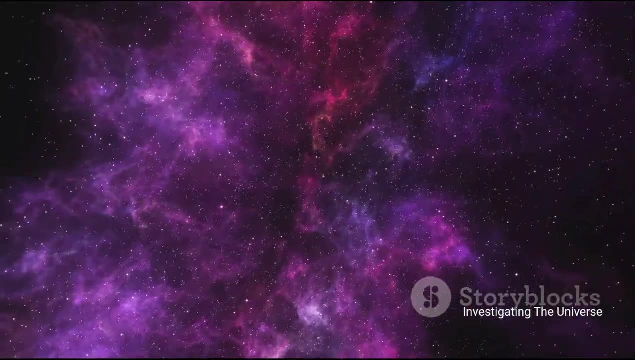 structures. they're not simply random, but rather they seem to follow a pattern beyond the physical body. we understand what causes them. in our everyday life we that repeats at different scales, just like a fractal. the second piece of evidence comes from something called cosmic microwave background radiation. this is a faint glow of heat that 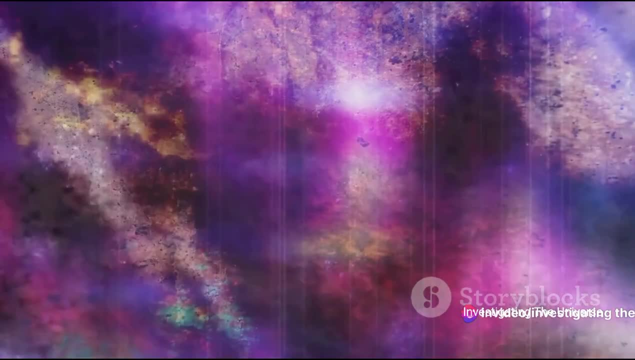 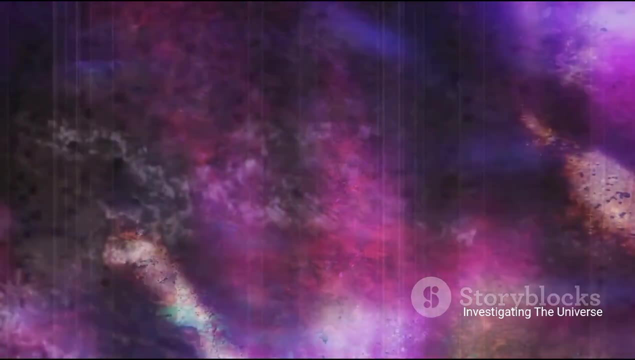 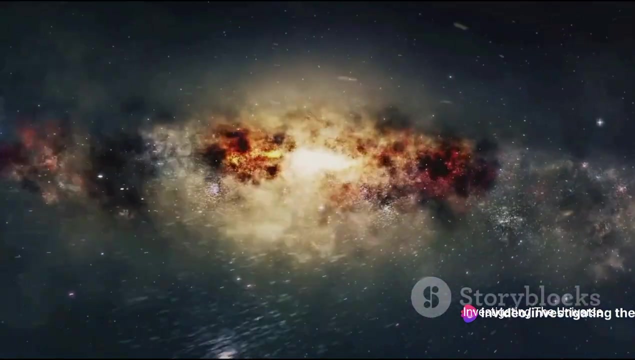 pervades the entire universe, a relic from the big bang itself. it's remarkably uniform, but upon closer inspection, there are tiny fluctuations in temperature. these fluctuations, when mapped out, also appear to follow a fractal pattern. now, this doesn't mean that the universe is definitely a fractal. there are other explanations for these observations. 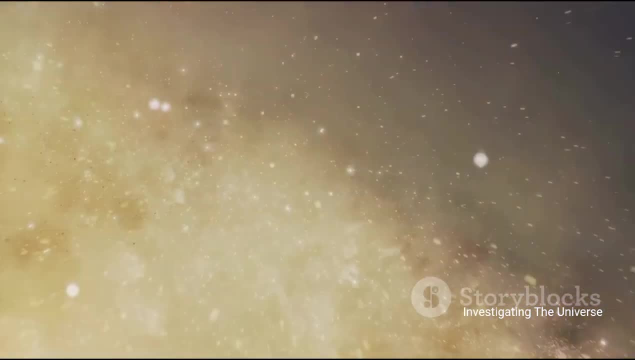 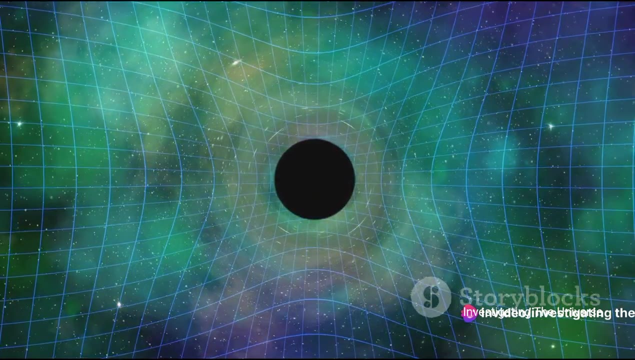 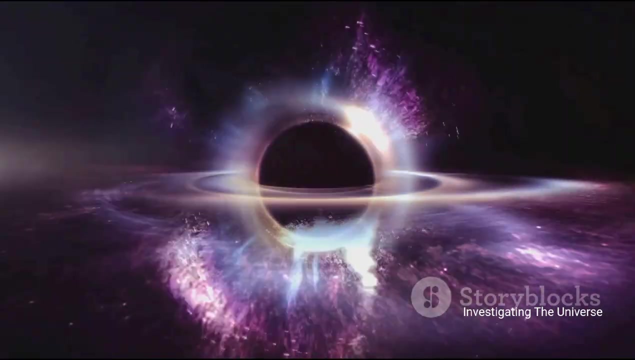 for example, the large-scale structure of the universe might be due to the gravitational pull of dark matter, an invisible and mysterious substance that makes up about 85 percent of the matter in the universe, and the fluctuations in the cosmic microwave background radiation might be due to quantum fluctuations in the early universe magnified to cosmic. 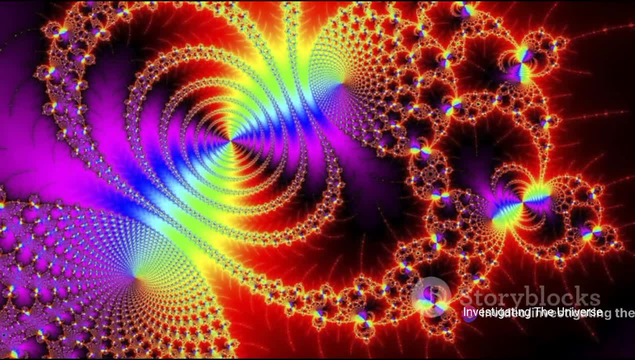 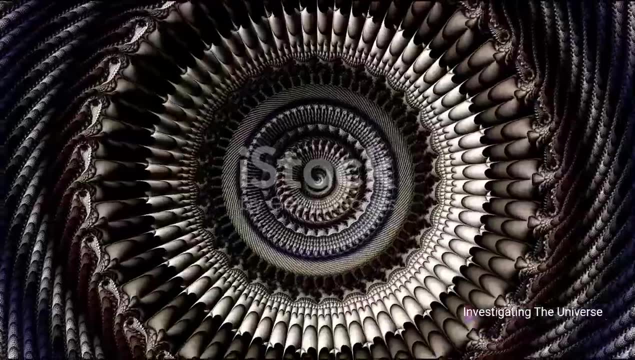 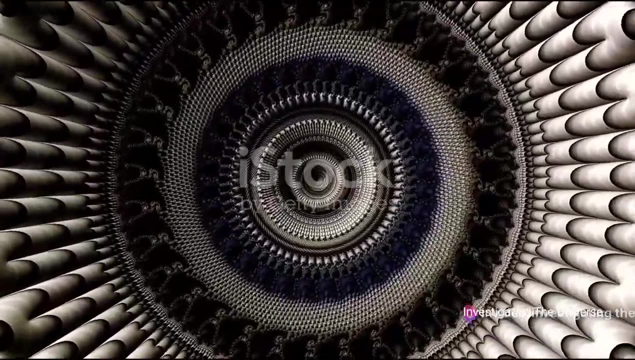 scales by the expansion of the universe. universe, However, the fractal universe theory provides a compelling explanation for these observations. It presents a picture of the universe that is both infinitely complex and beautifully simple, A universe where the same patterns repeat at all scales, from the tiniest. 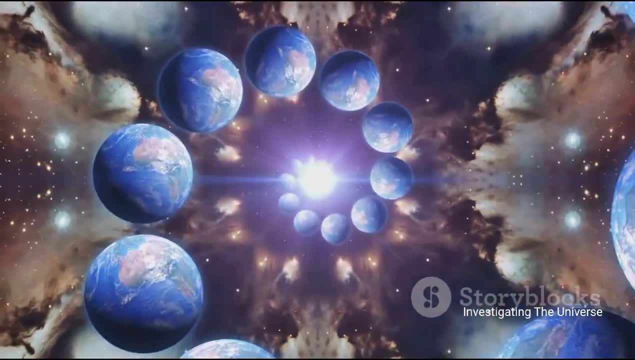 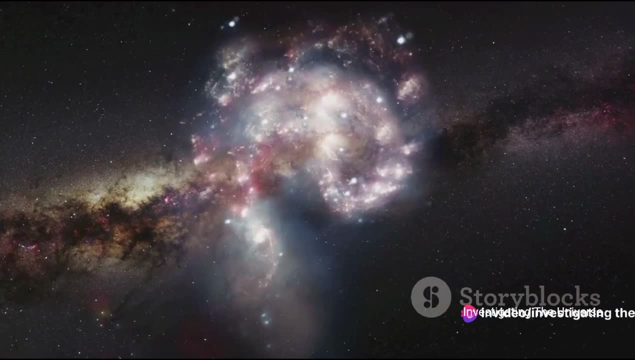 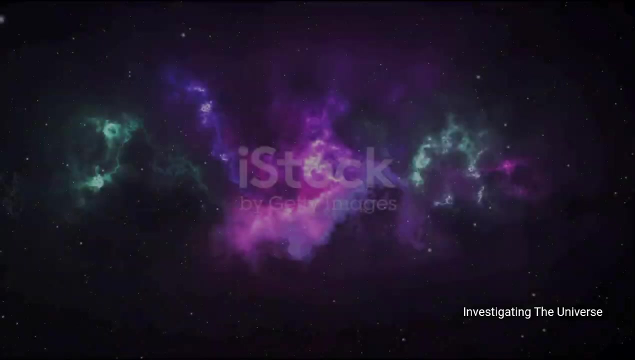 particles to the largest cosmic structures. Though it's a compelling theory, it's not without its criticisms. But as we delve deeper into the mysteries of the universe, the fractal universe theory continues to provide intriguing possibilities for our understanding of the cosmos. Like every theory, the fractal universe theory has its critics. As we delve into the criticisms, 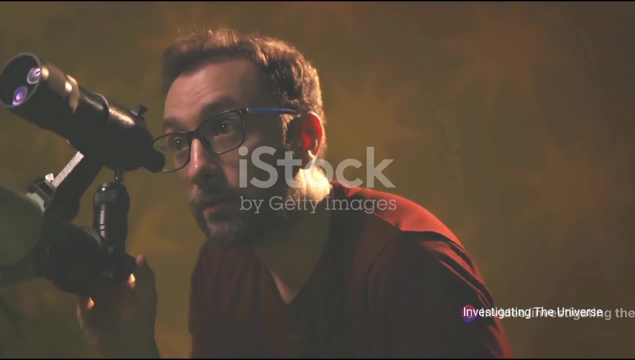 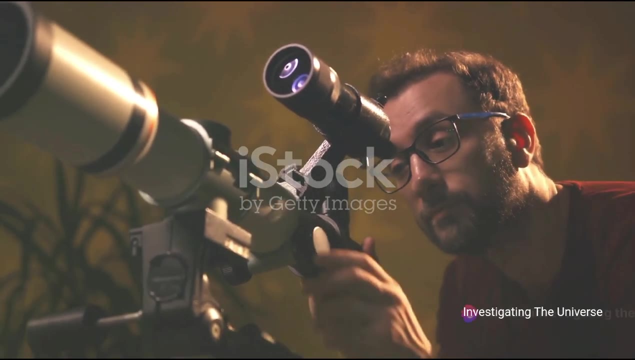 of the fractal universe theory, we find two primary areas of contention. First, we encounter the limitations of our observations. As it stands, our current technology only allows us to gaze so far into the universe, as if we were in the middle of the universe. But as we delve deeper into the 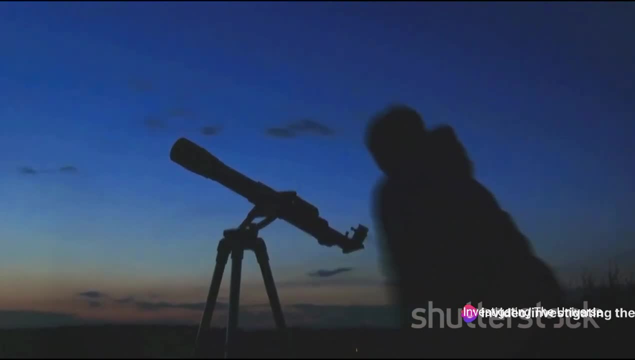 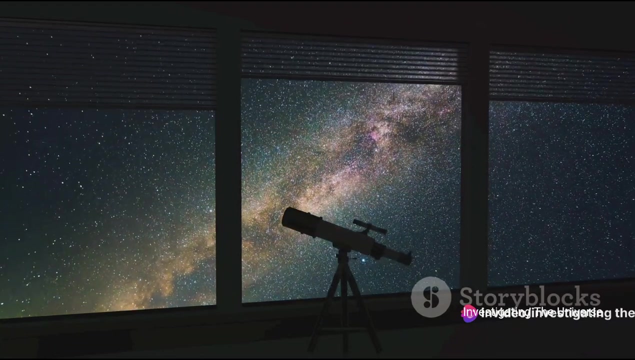 cosmos, we are restrained by the finite speed of light and the size of the observable universe. Consequently, we cannot directly observe the entirety of the universe and confirm whether its structure is truly fractal in nature. Critics argue that our inability to test this aspect of 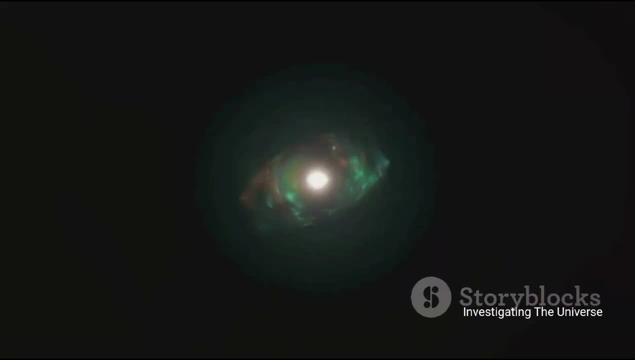 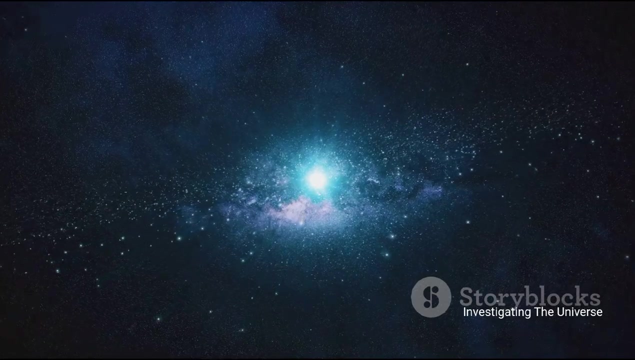 the theory limits its scientific validity. Secondly, the fractal universe theory has implications for the widely accepted Big Bang theory. The Big Bang theory is a theory that suggests a universe that began from a single point and has been expanding uniformly ever since. This results in a homogenous and isotropic universe on a large scale, a viewpoint that 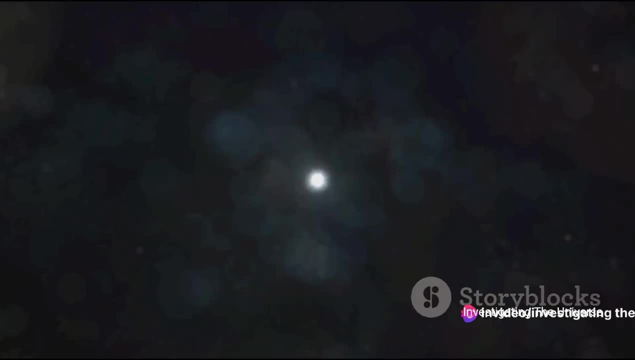 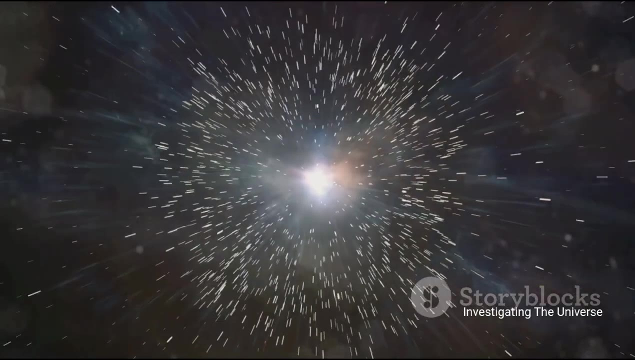 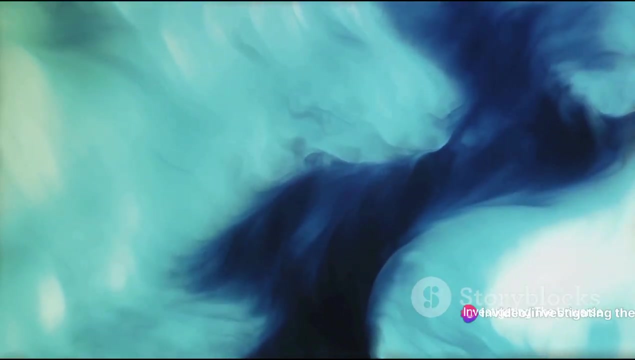 doesn't gel well with the idea of a fractal universe. Critics argue that the fractal universe theory, with its infinite repeating patterns, contradicts the Big Bang's concept of a universe with a definite beginning and a uniform expansion. Moreover, critics point out that the fractal universe 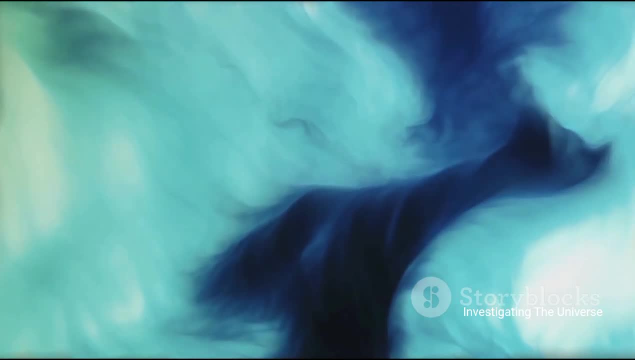 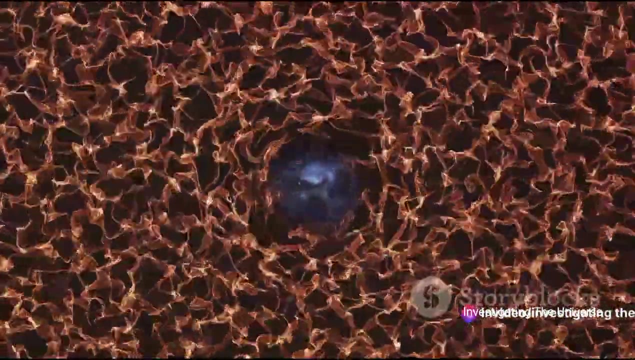 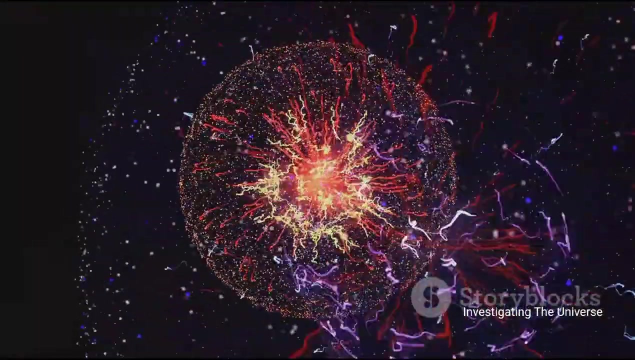 theory does not align with the cosmic microwave background radiation data. This radiation, a remnant from the Big Bang, is extremely uniform across the universe, which is more consistent with the Big Bang theory's predictions than the fractal universe theories. And let's not. 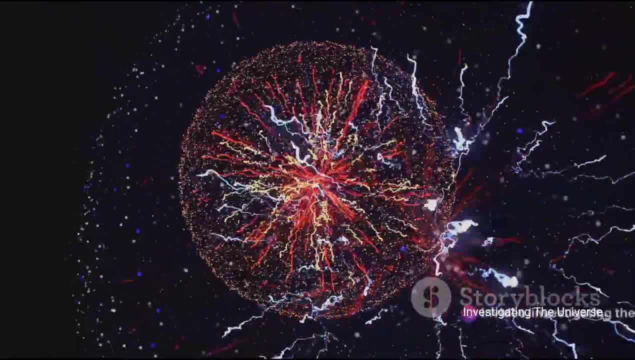 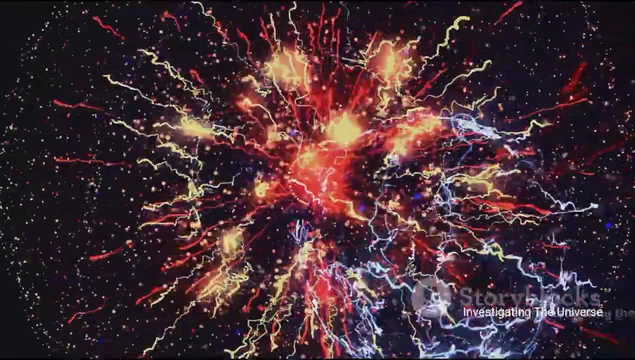 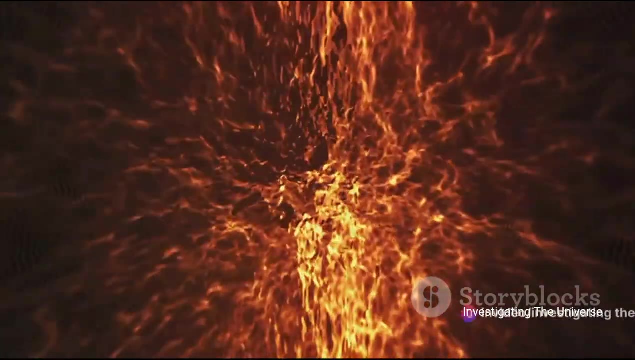 forget the role of dark matter and dark energy, which together make up approximately 95% of the universe. Their existence and behavior have been inferred from their gravitational effects, But how these elusive substances fit into the fractal universe theory is still an open question.